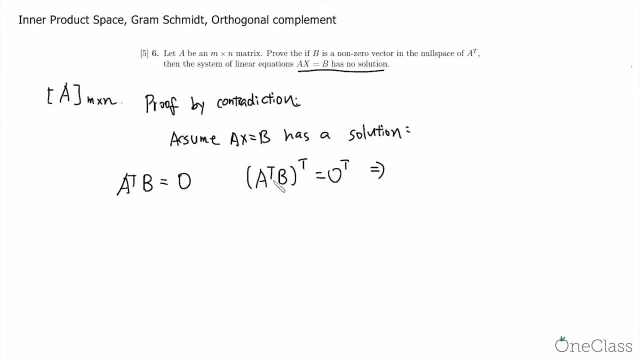 transpose, to put this transpose into the bracket. but we have to switch the position of the first and second element. So we have B transpose, A transpose. transpose equals to 0, since 0 transpose is still 0. And we try to simplify this a bit- We have B transpose, A equals to 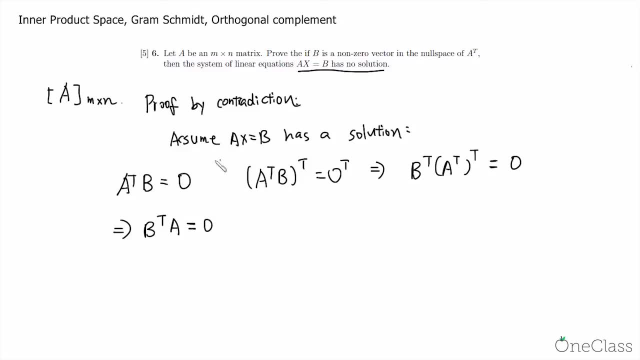 0. And now we know we have made the assumption that AX is equal to B. There's a solution. Therefore this equation holds. So now we try to multiply both sides by B transpose And we get B transpose. AX equals to B transpose B. And we know that B transpose A is 0. So 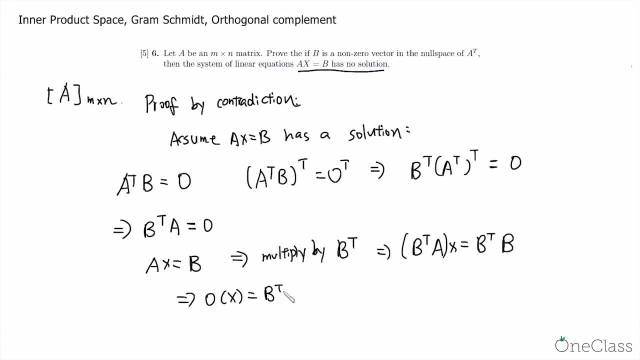 we know, 0X is equal to B. transpose B, which then gives us B transpose B is equal to 0.. And one fact that we need to know for this proof is that if we have any vector X1 to Xn and we multiply it by its transpose X1 to Xn, what we get is X1 square plus dot dot. 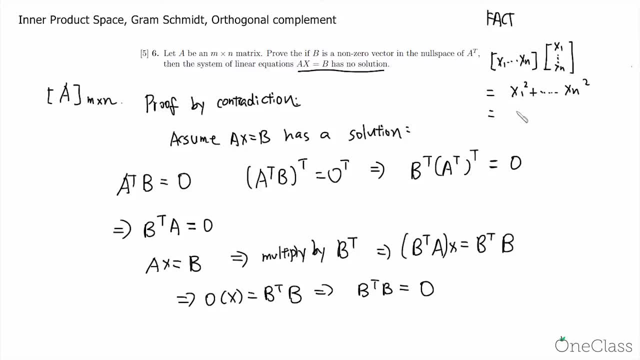 dot Xn square, which is the same as X1 to Xn in the product itself, which is then equal to the length of X1 to Xn square. So in this case, since B transpose multiply B equals to 0, then B transpose multiply B is also equal to B. length square equals to 0.. And the length 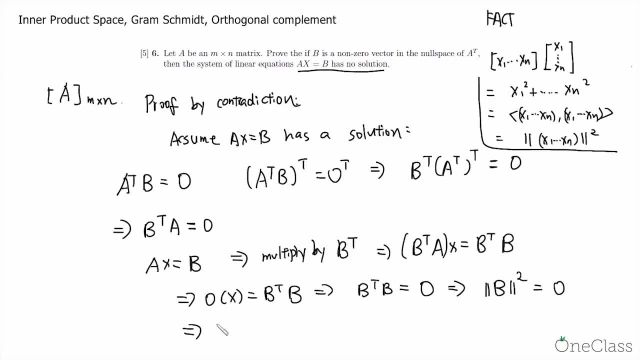 of B square is only 0 when B is 0. And that is given in the definition of inner product. The inner product of the same vector will be 0 only if the vector is 0. So in this case, B length square is equal to 0 only if, and only if, B is equal to 0. And this is a huge contradiction. 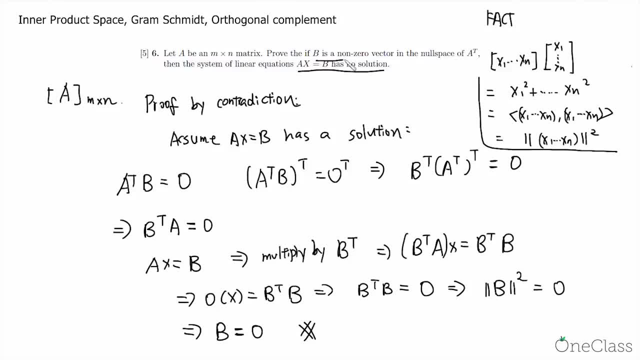 because in the question we are given that B is non-zero vector. So we have a contradiction, since B is non-zero vector, So we have a contradiction since B is non-zero vector- 0, 0,, 0, 0, and if we make the assumption that Ax equals to B has a solution, then we